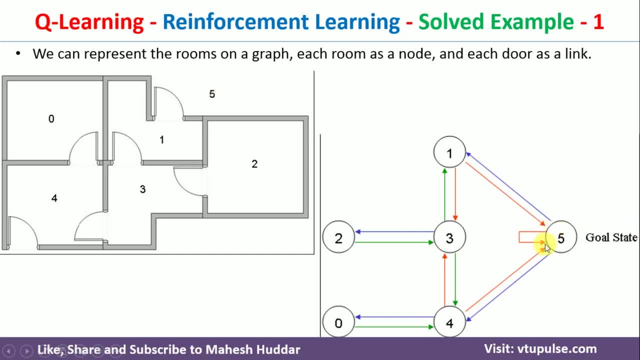 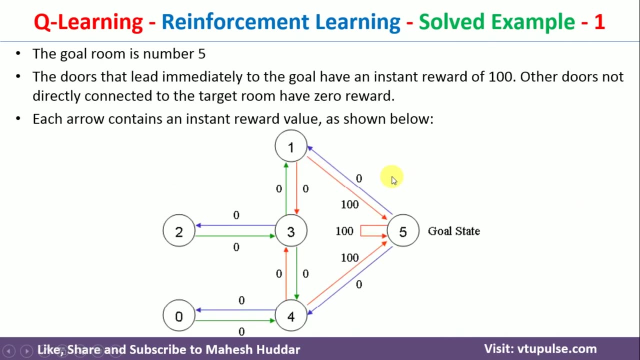 go from 5 to 5 over here. So that is represented here. So in this case we assume that 5 is the goal state here. So we need to identify an optimal path from each and every state to this particular goal state over here. And one more very important thing we need 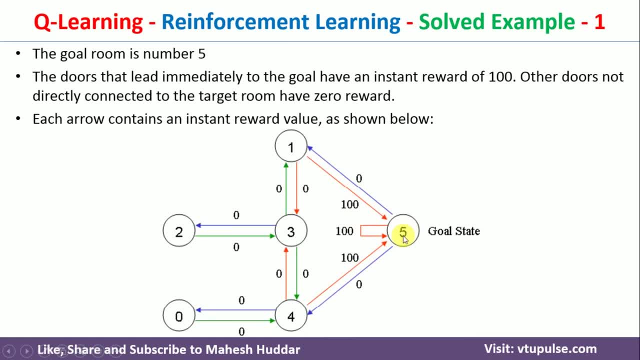 to remember is an action which will lead to this particular goal. state will get an instance reward of 100 here, Remaining all are 0 in this particular case. So this is the one action, This is the second action and third action which will lead to this particular 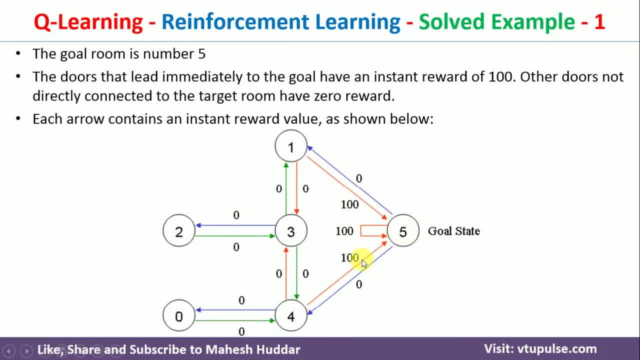 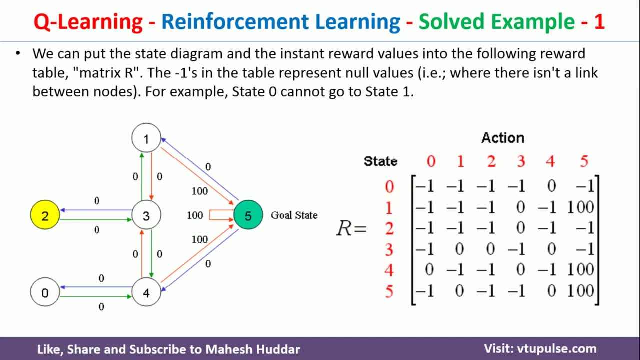 goal state. So each and every action is given an instance reward of 100.. Remaining all are 0 in this particular case. Now what we try to do is we will try to apply the Q learning algorithm to this particular can say that: 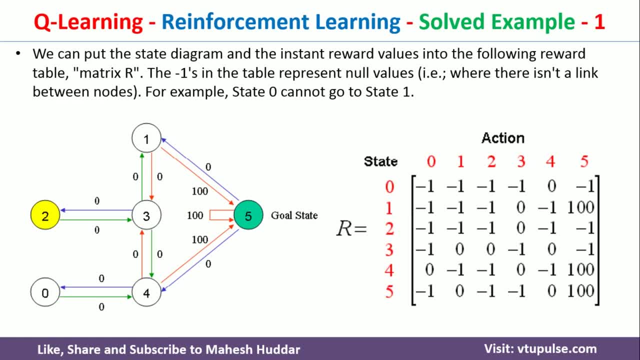 state diagram to get the optimal path over here. So the very first thing, what we need to do is we need to write the reward matrix. The reward matrix contains the states as the rows and action as the columns over here. In this case, we have six states, namely 0 to. 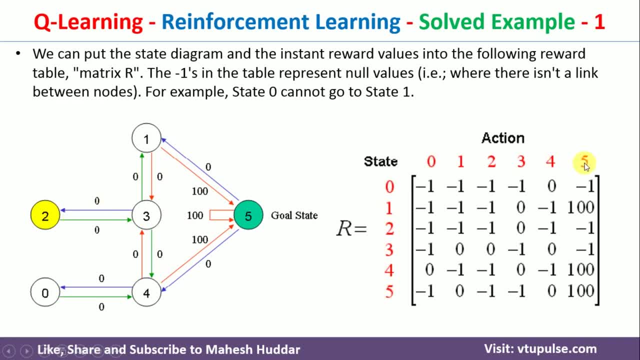 5. Actions are again six here, namely 0 to 5 in this case. Now I will show you how to put, now fill this particular reward matrix. Let us assume that you are present in state 0. When you are present in 0,, you can perform only one. 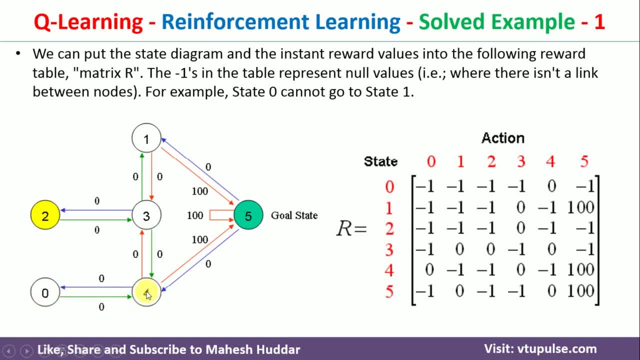 action, that is, this is the action which will go to state number 4.. That is, when you are present in state 0, you can perform an action 4, and then what is the reward? over here, that is 0, remaining all are minus 1 in this case. So from this particular row, you can understand. 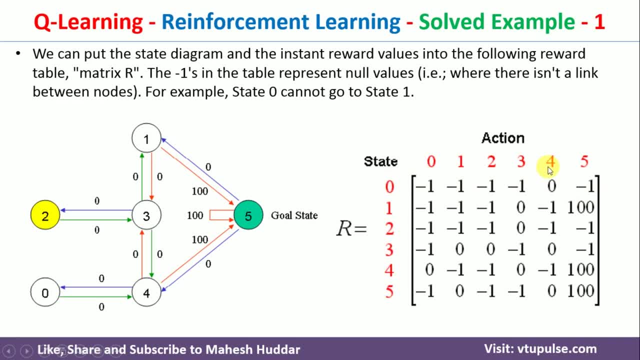 that when you are present in state 0, you can perform an action 4.. Then you can perform only action 4 over here. Similarly, I will talk about this particular second row- When you are present in state number 1, you can perform an action 5 here, or you can perform: 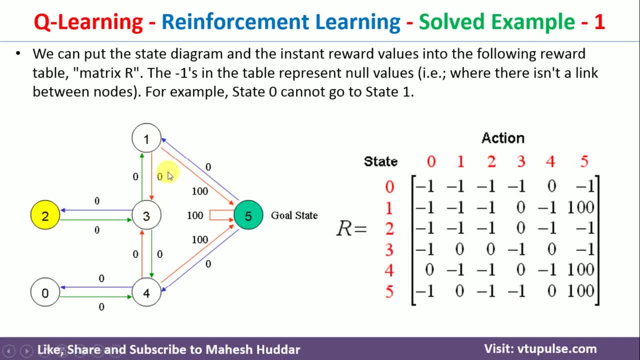 an action 3 here. If you perform an action 3, the reward is 0.. If you perform an action 5, the reward is 100 here. So, when you are present in 1, if you perform an action 3,. 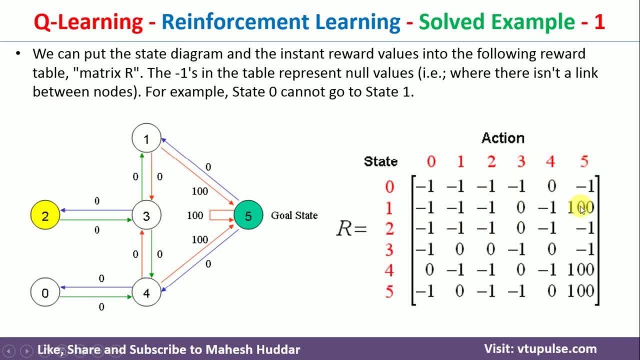 the reward is 0.. If you perform an action 5, the reward is 100. here, Similarly, we have to fill this particular entire matrix here. Minus 1 indicates there is no direct edge between that particular states over here. Now this algorithm I have discussed in detail. 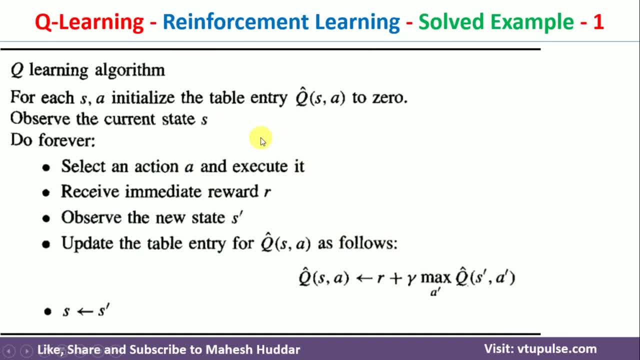 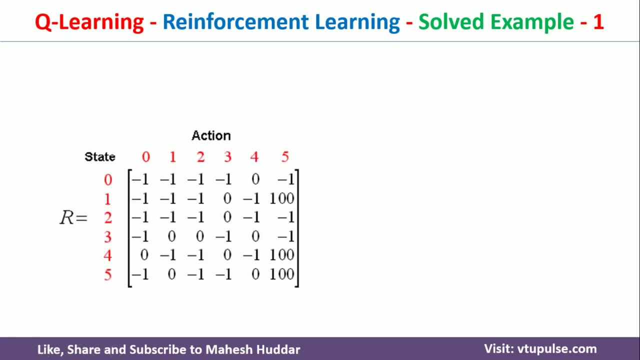 in the previous video. The link for that particular video is present in the description below. Go through that particular video so that you can understand the Q-learning algorithm in detail. That will help you to understand this particular example over here. Now coming back to the next part of this particular algorithm. 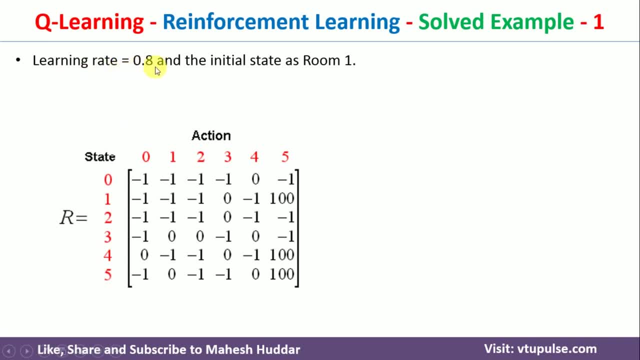 The very first thing. what is required is we need some learning rate. I will initialize it to 0.8.. We need to start from one initial state. I will consider the initial state as 1 over here, And then we need to initialize the Q-matrix. over here, The Q-matrix is initialized. 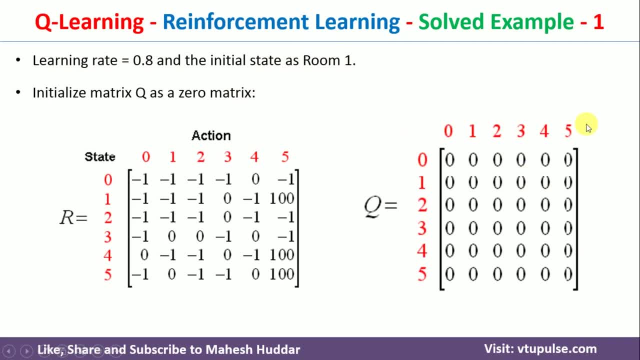 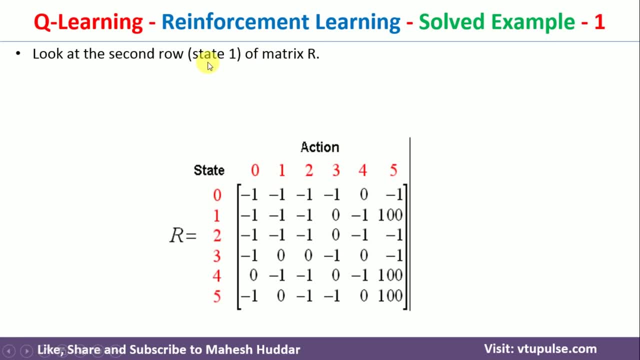 to 0 initially, So we have put 0 for every state and action in this particular case. Now what I do is I will consider the initial state as 1.. As I said earlier, we will start with the initial state as 1.. 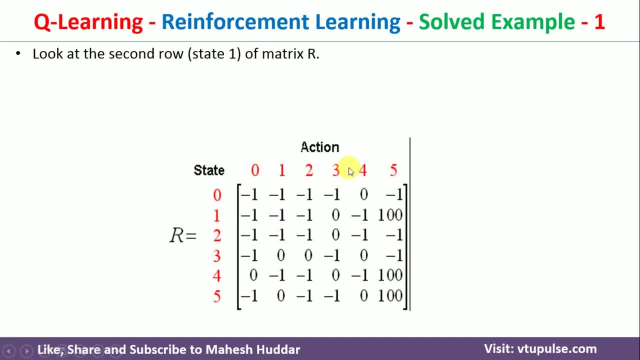 Because initial state is 1, we can perform two actions over here. Either we can perform 3 or we can perform 5 here. So if you perform 3, you will get the immediate reward of 0. And if you perform an action 5, you will get an immediate reward of 100 here. So between 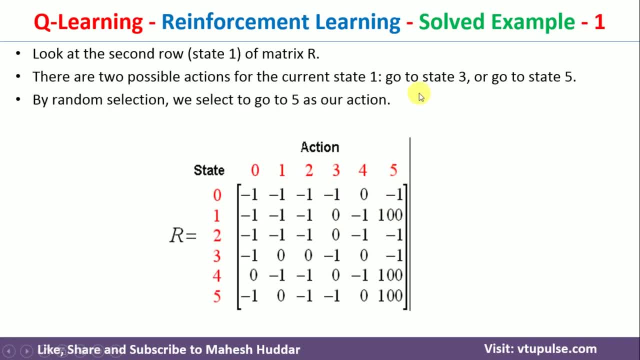 these two. we need to select one action here. Let us assume that I will select an action 5 in this case. If I select an action 5, I will get the immediate reward of 100 in this case, And the next state will become 5 over here. 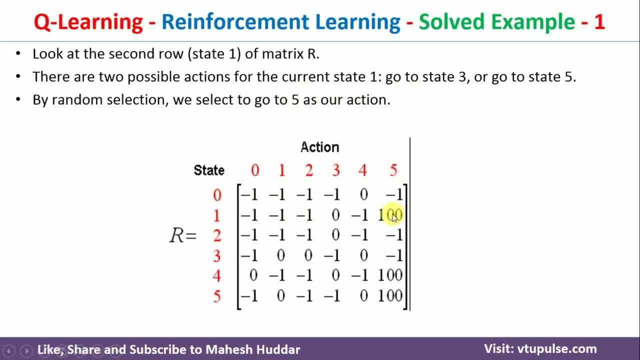 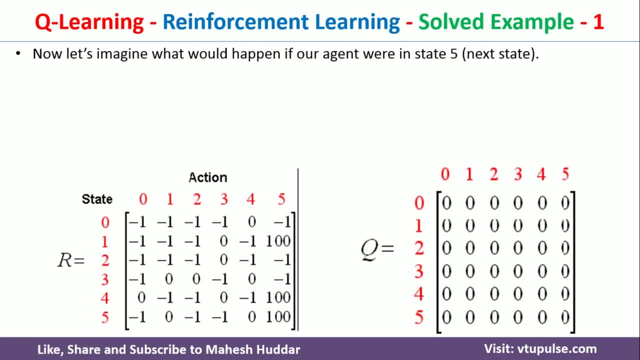 So the current state is 1 and the next state is 5. And the immediate reward in this case is 100 over here. Now, when you get this particular next state as 5, we need to identify what all things we can perform when we are present in the next state- 5 over here. So what all things? 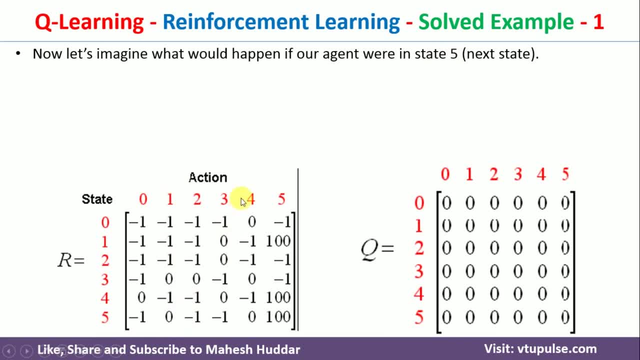 you can perform. You can perform an action 1 because here it is 0.. You can perform action 4 because it is 0 here. You can perform action 5 here, because it is 100. here You cannot perform any other things, because when you are present in the next state, you will get. 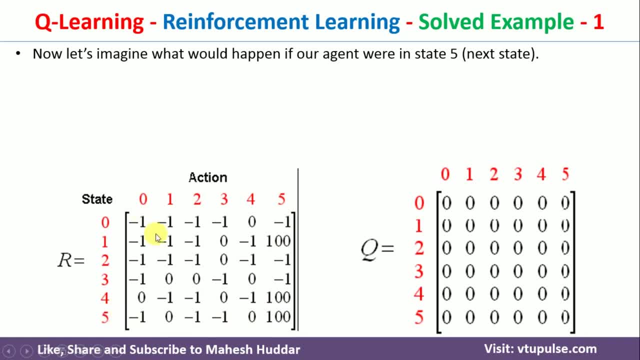 an immediate reward of 100 over here, So you can perform an action 0 because it is minus 1 over here. You can perform 1, or you can perform 4, or you can perform 5 in this case. So now we know the Q learning equation, that is Q of current state comma action Current. 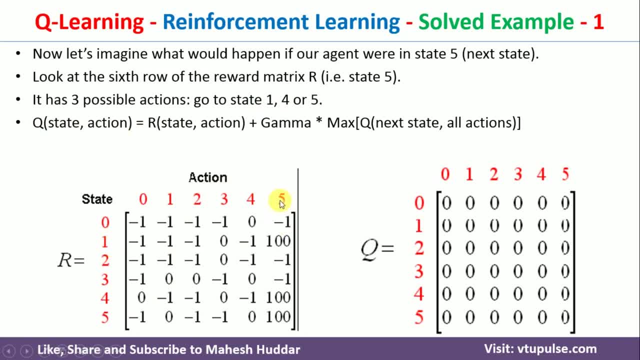 state is or initial state is 1 comma action. what we have selected, 5, that is the action over here. R of state comma action. state is 1, action is 5 here. So R of 1 comma 5 is how much 100.. So that will become over here. Gamma is the learning. 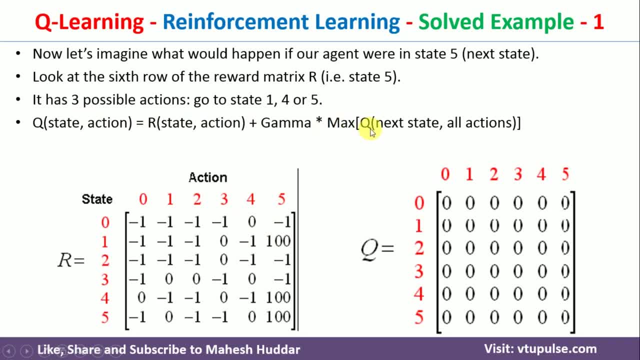 rate multiplied by maximum of very important point. Q of next state comma: all actions. What is the next state? we have selected 5 here. What are the actions we can perform? You can perform 1,, 4 or 5.. So you have to put it over here Now. Q of 1 comma, 5, R of 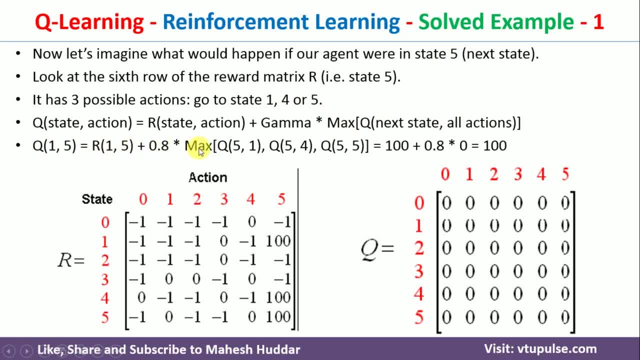 1 comma, 5 plus 0.8, that is a gamma maximum of Q of next state, that is 5.. What all actions you can perform, First time 1, second time 4,, third time 5 here. So this particular. 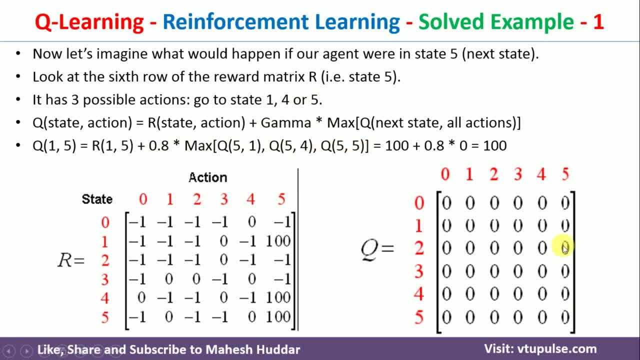 5 comma 1,, 5 comma 4, 5 comma 5. in this particular Q matrix. everything is 0 here. So maximum of 0 is 0. multiplied by 0.8 is 0.. R of 1 comma 5 is how much R of 1 comma 5 is equivalent. 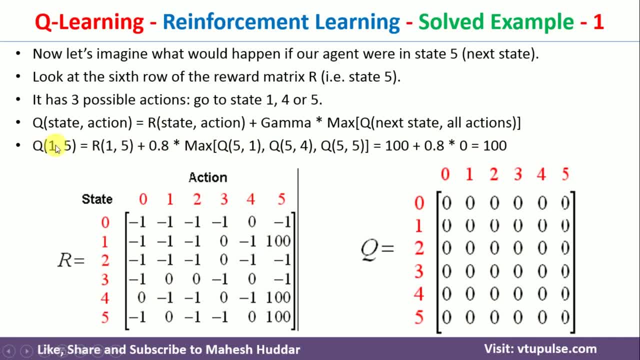 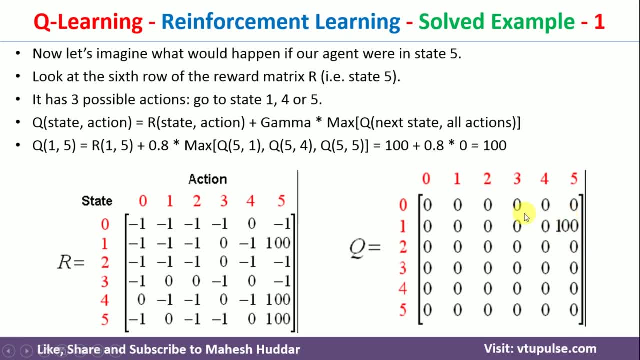 to 100. So this will become 100 in this case. Q of 1 comma 5, 1 comma 5 will be 100 in this particular case. So that is what you can notice in this case. Now, what has happened here is when we were present in this particular initial state 1. 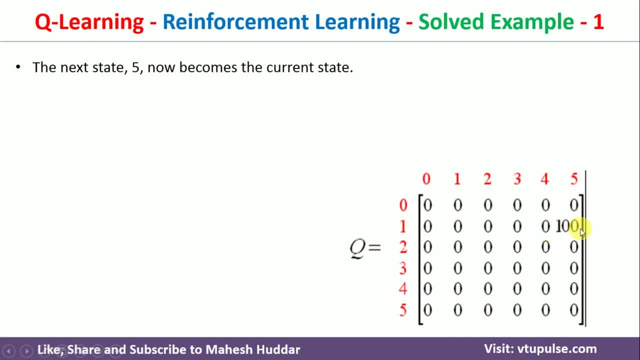 and after applying that particular Q learning algorithm, we have reached to the goal state here. Because we have reached the goal state, one episode has finished. Now we need to perform the same set of episodes for each and every initial states over here. Now what? 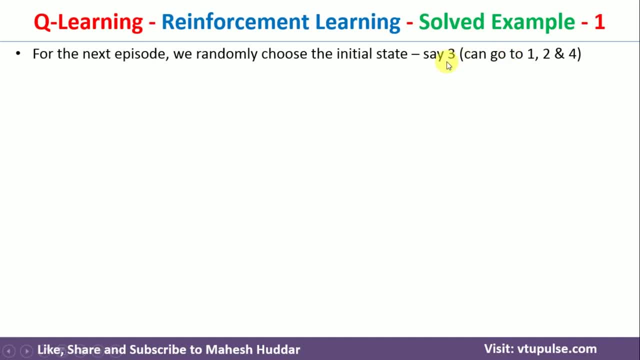 I will do is I will consider the initial state as 3 for the next episode. So if I consider 3 as the initial state, I will consider the initial state as 3 for the next episode. So if I consider 3 as the initial state for the next episode. you can see here you can perform. 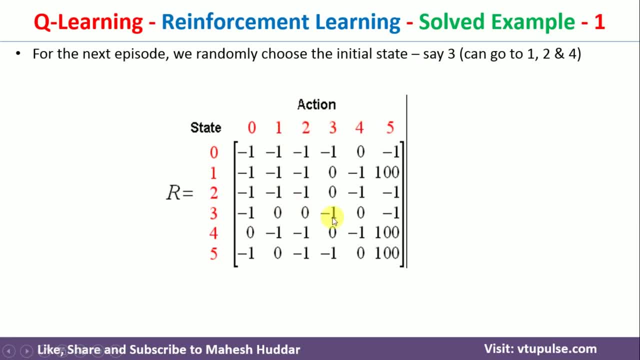 an action 1 or action 2 or action 4, because we have some values here Remaining. all are minus 1.. So we cannot perform those particular actions. That is what I have written here. Now, between these three, we need to select one action. Let us say that I will select. 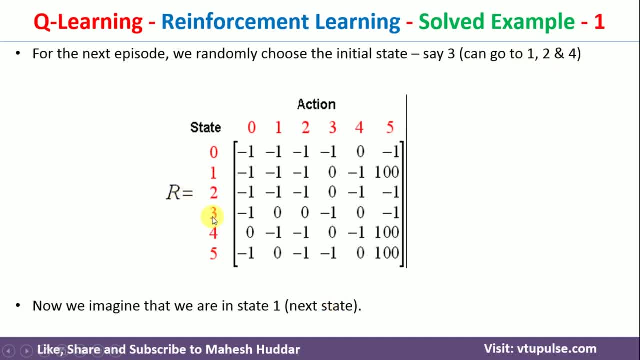 action 1 in this particular case. So the current state or the initial state is 3 and the next state is equivalent to 1 in this particular case, From the initial state to 1, we got the immediate reward is 0 in this case. This is one more important point. we 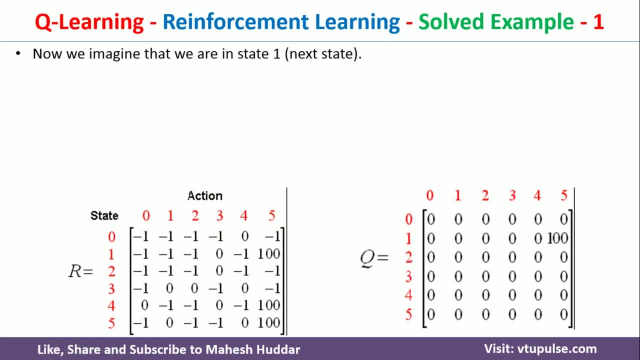 need to remember here Now, once you select one as the next state, what all things you can perform. you can perform an action 3 or you can perform an action 5 over here. So those are the two things you can perform here. We will put those party things in the equation. 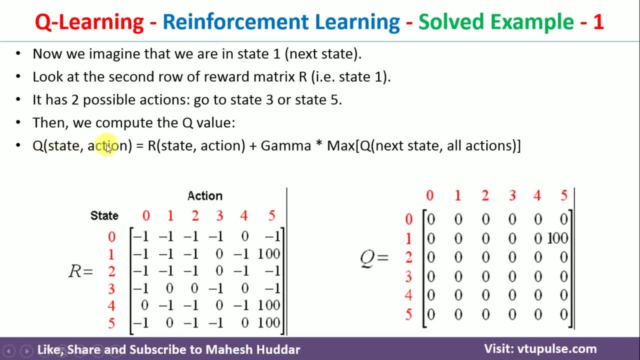 again, If the initial state is 3, and the action we have selected is 1, that means Gamma of maximum 1, isasse- What is the next state? The next state we have selected as 1, what all action you can perform is 3 and 5 over here. so if you put all those things in this, 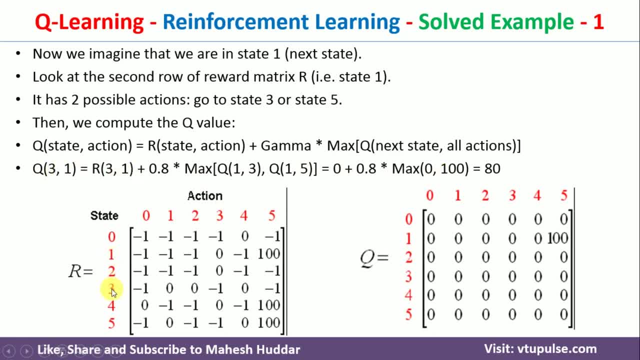 equation that is: 3 comma 1. r 3 comma 1. what is r. 3 comma 1, 3 comma 1. what is the value here? 0. so that is what i have written here: 0.8 is the gamma value max. max is nothing but max of this particular. 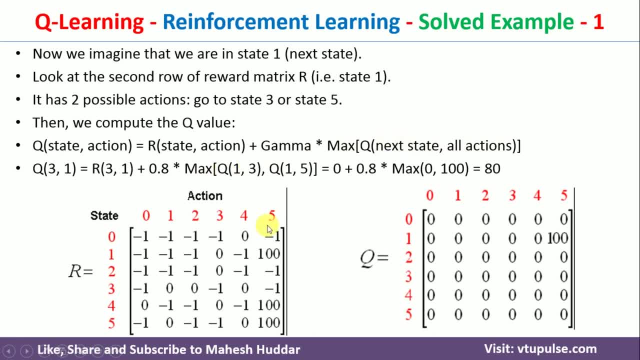 part. so max of q next state is what next state? we have selected 1. what are the actions you can perform? 3 and then 5 over here. so 1 comma 3 and 1 comma 5. 1 comma 3 is how much 1 comma 3 is. 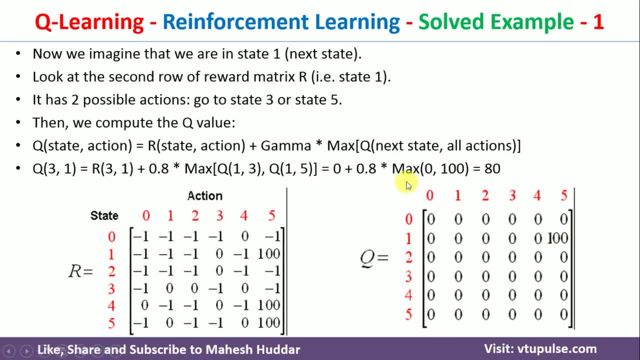 equivalent to 0. 1 comma 5 is equivalent to 100 here, so 0 and 100 between these two. what is the maximum that is 100 here? so 100 multiplied by 0.8 is 80, and this particular part is already 0, 3. 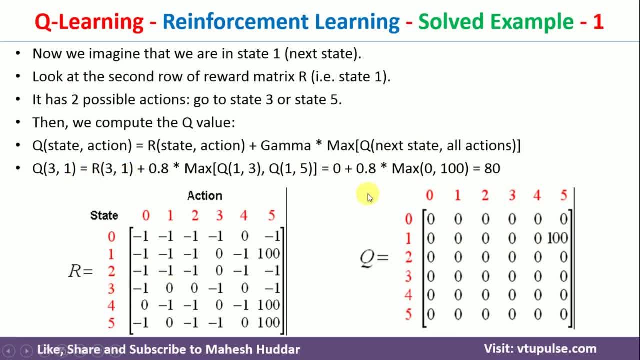